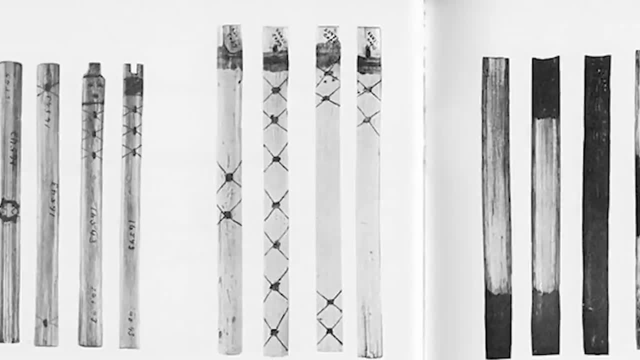 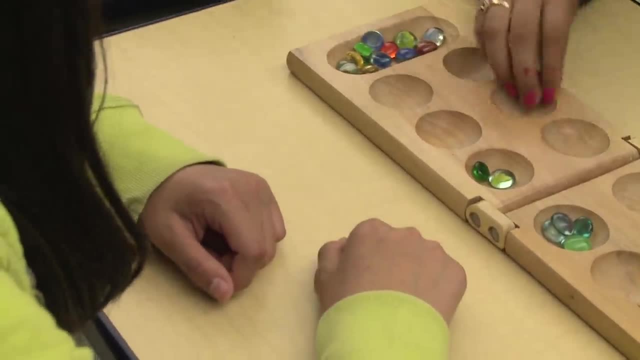 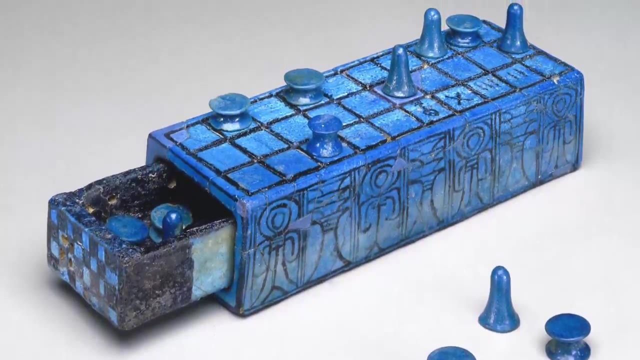 With the earliest form of dice being knuckle bones and etched sticks which can be rolled for a random number or divination. Early stoned etched mancala boards can be found in prehistoric Africa. Board games quickly become more complex and ornate in their designs and rule sets, as games like Senate can be found in Egypt. 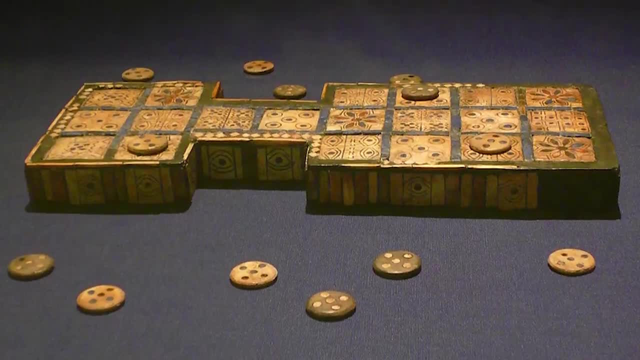 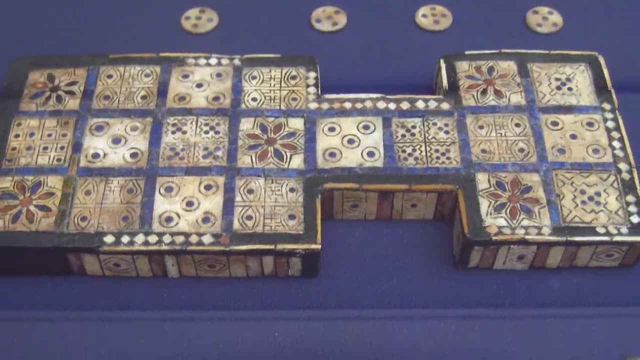 In Ur, modern-day Iraq, The Royal Game of Ur and Proto-Chequers are popular in 2600 BCE. The Royal Game of Ur was another racing-style game which was superseded by backgammon in style and popularity around 2000 BCE. 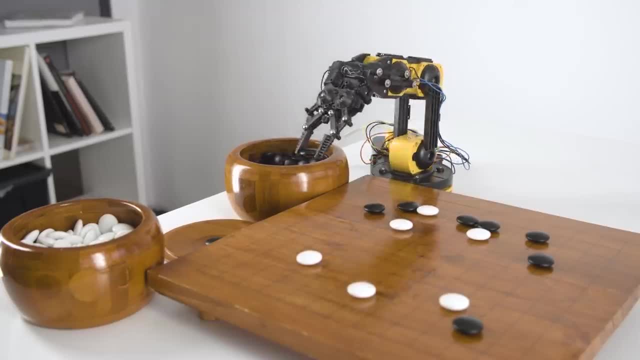 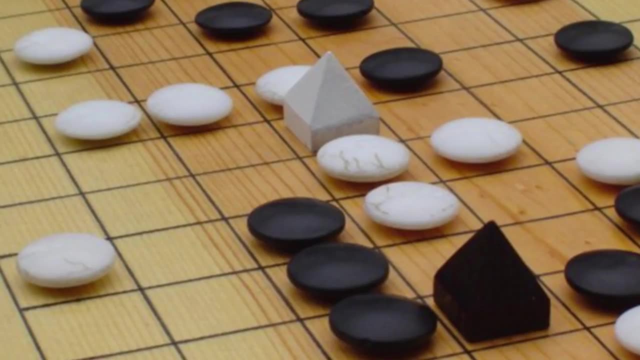 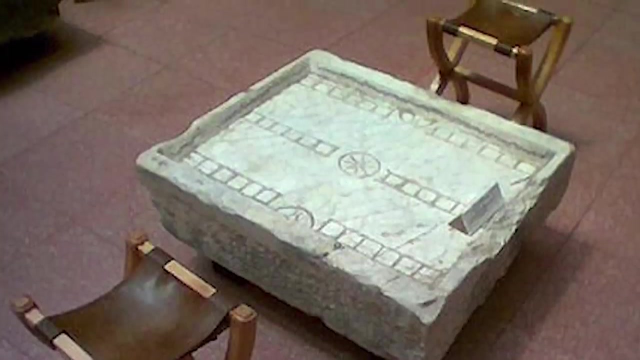 Meanwhile, in China, people were playing Go, a high-strategy territory capturing game. In 1300 BCE we find Laetus Latruculurum- Laetus Latruculurum and the Roman Empire, A two-player strategy war game which is believed to be a prototype of chess. 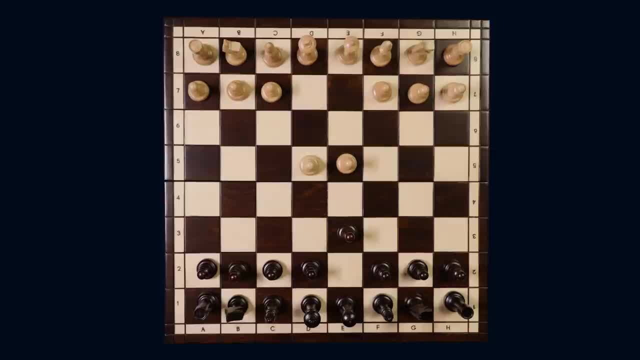 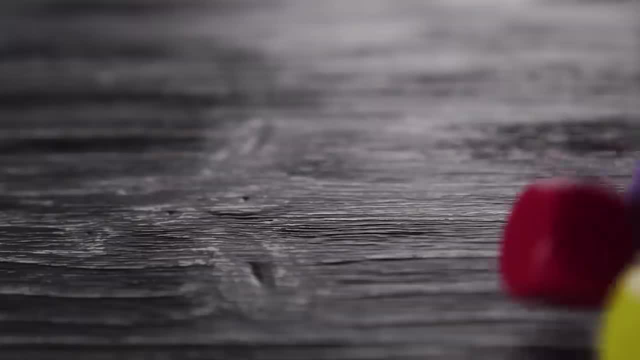 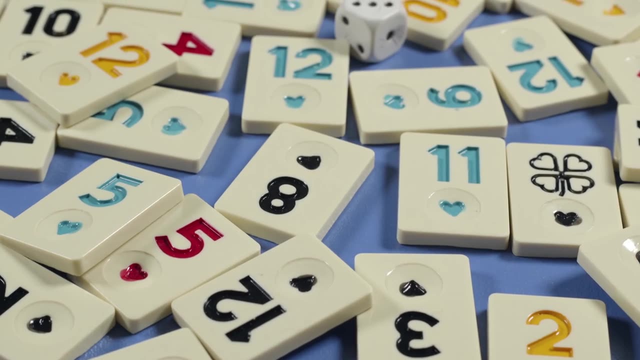 There are many versions of chess which are found across the ancient world, until Mad's Queen Chess became a popular variant in the Middle Ages, which is the same version of chess that we play today. In today's board games, the table-chop genre is coming back stronger than ever, with advancements in game design and the ability to produce large amounts of intricate pieces very quickly and cheaply with plastic and cardboard. 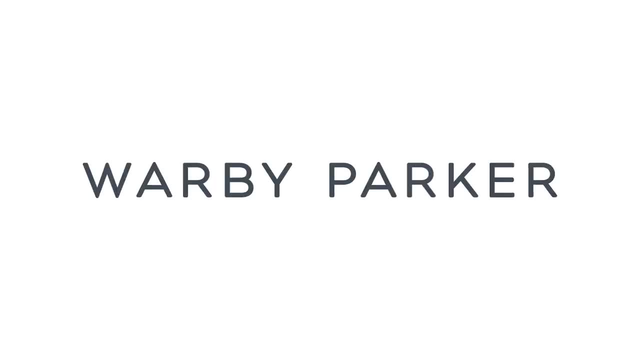 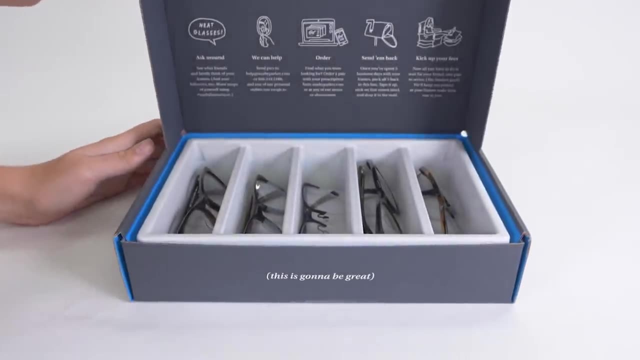 But before Adam starts making the game. this video is sponsored by Orby Parker is committed to providing exceptional vision care online and in stores, offering eyeglasses, sunglasses, eye exams and contact lenses. Glasses start at $95, including prescription lenses, sunglasses, progressives and blue light lenses are also available. 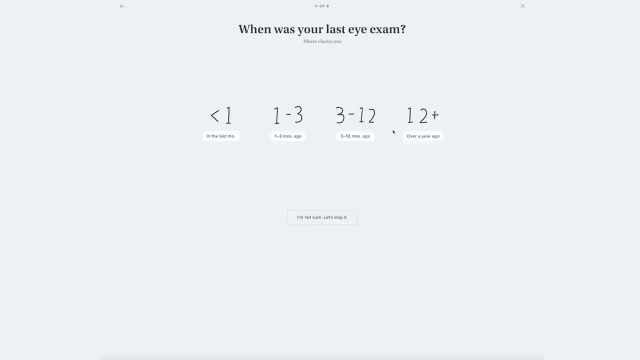 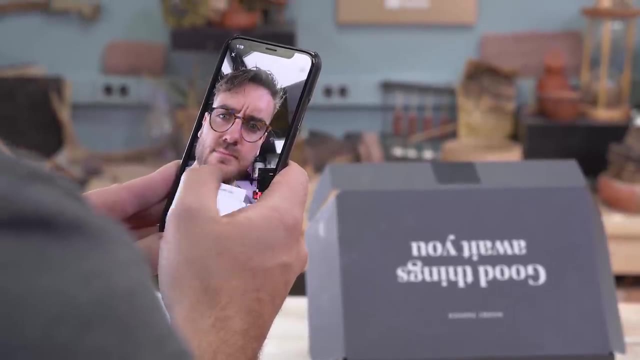 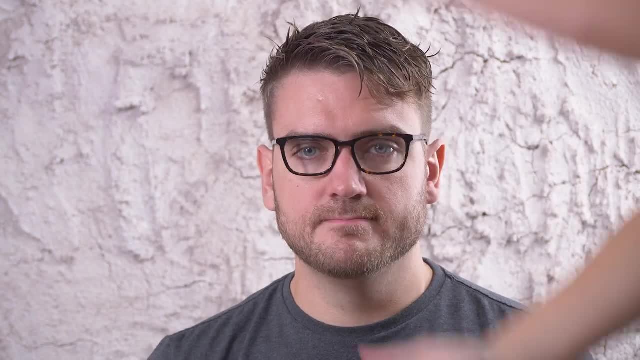 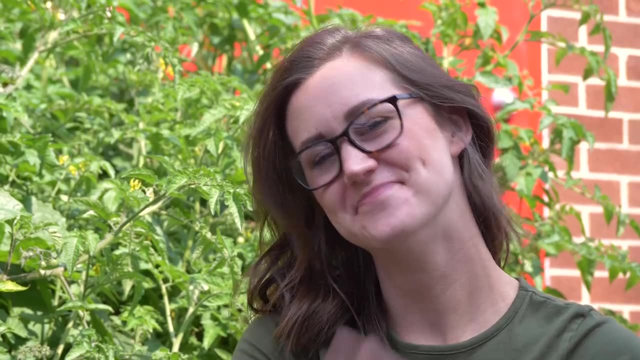 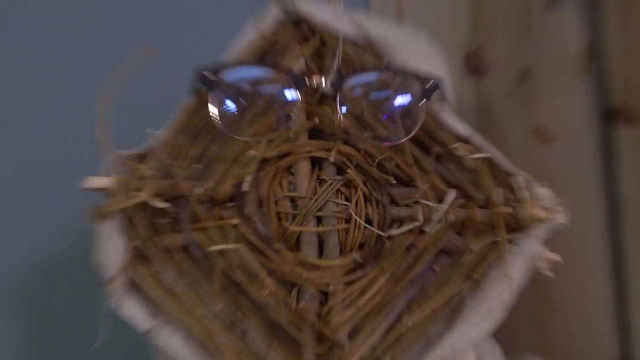 And see what was the best. look for me. Ships free and includes a prepaid return shipping label. Their styles range from extra narrow to extra wide, so they can fit pretty much any face shape. Try five pairs of glasses for free at home at warbyparkercom slash htme. 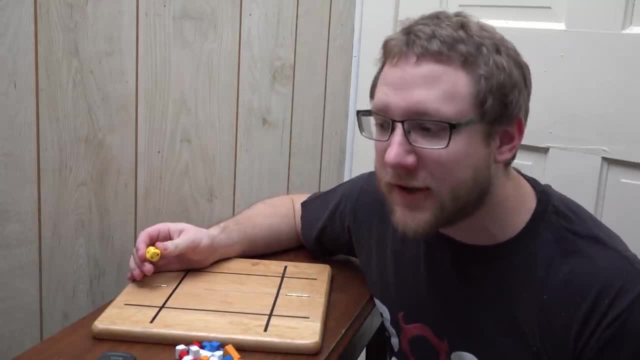 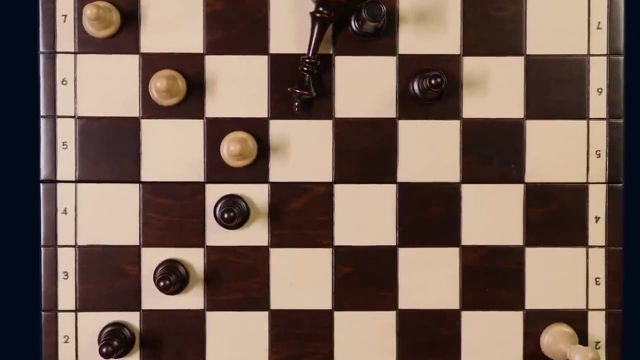 Let's talk about designing a game. So when I first got into this stuff it really kind of struck me- Mechanics are what they call the pieces of a game that kind of create the fun. Mechanics and design sounded like weird words to use when you're talking about making a game. 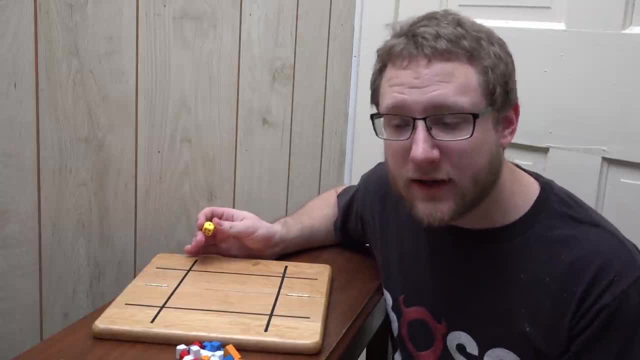 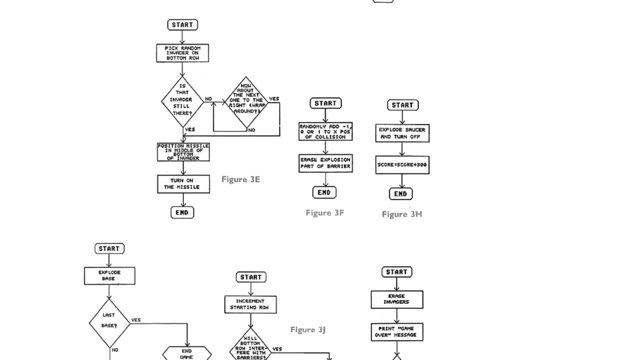 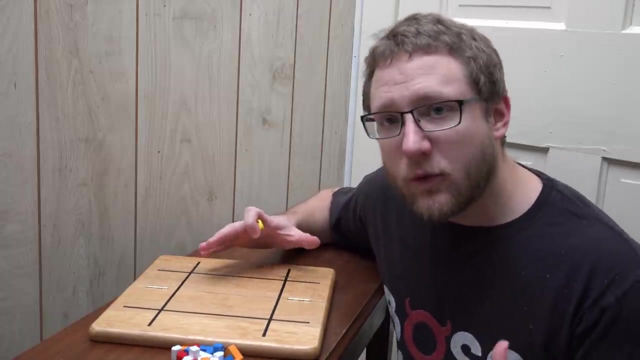 The truth is that games can actually be constructed very intentionally with designs, flows, loops, things that make play happen. What we need to do is we need some sort of a tabletop game. I've got limited materials, so I'm going to try to use some good rules and constructions. 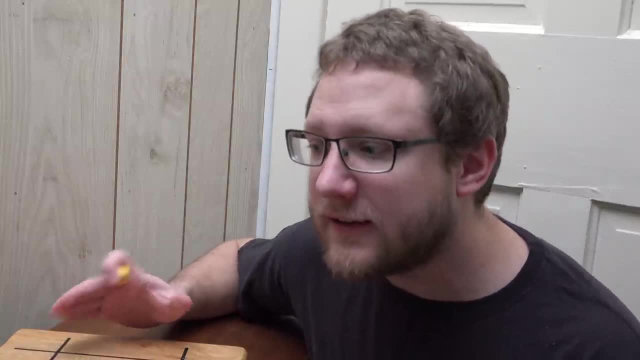 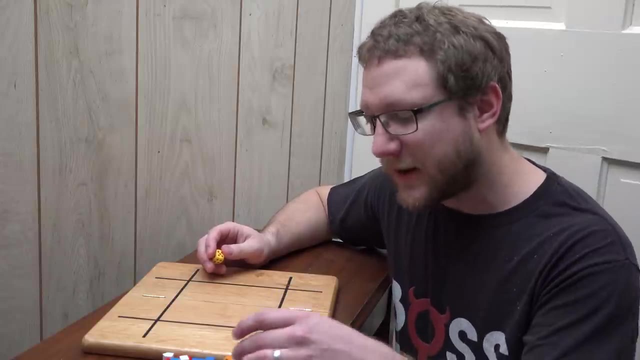 Create a game that is going to be fun and enticing, replayable, has some strategy to it but, at the same time, a little bit random. A very popular thing to do with games is to make a race game, And with these race games, what you would do is you just have different pieces. 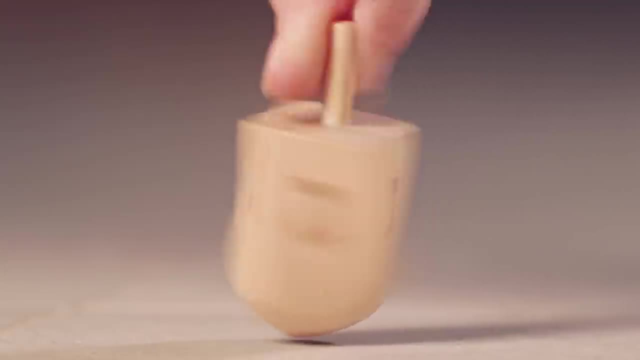 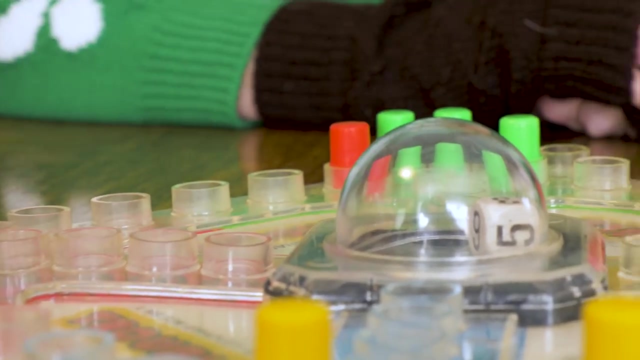 and you could just have a randomizer of some sort of spinner or top You roll and then you would go around the board: Whoever wins wins. That's trouble, The randomizer being colors, that's life. Random going up and down, that shoots some ladders. The Royal Game of the Goose is a. 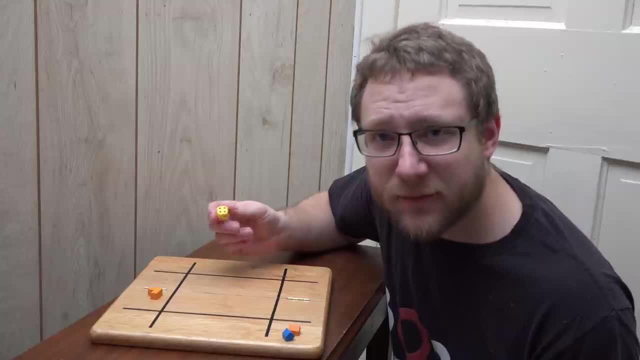 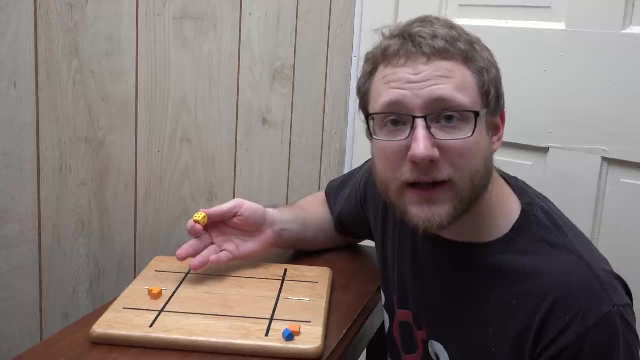 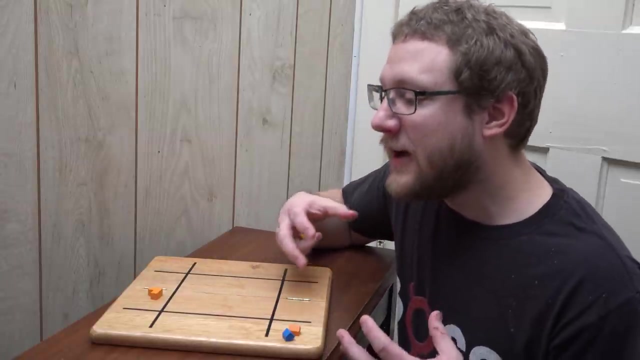 very popular historical game. Some race game can have some bits of strategy to them, And what lets you do the strategy, what lets it be more for a broader audience or a bolder audience, is unlike Uno or something you actually can control the game. You can actually play it and make decisions. 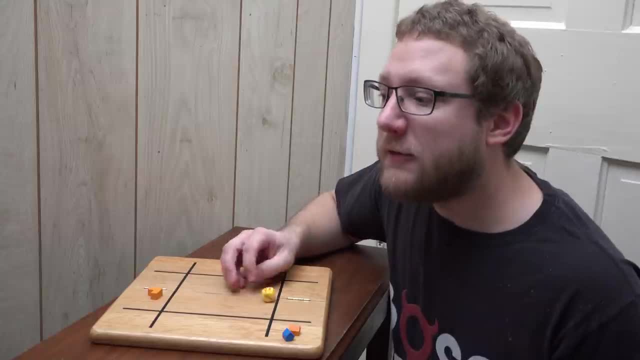 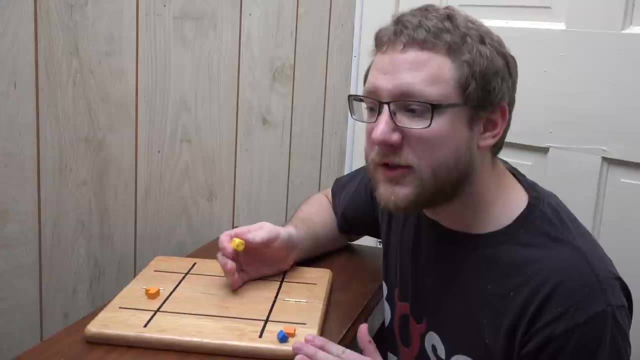 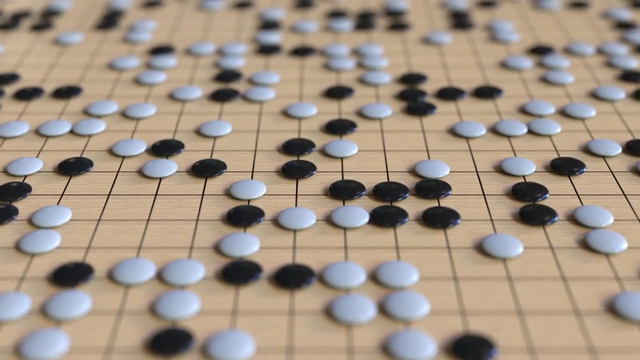 that influence it. So you can create a strategy. If you have a little bit of randomness, that can disrupt the strategy some and make you make counter plans, which is why randomness is a still used. If you have a game that is entirely without randomness, you can do that. Go, is that? 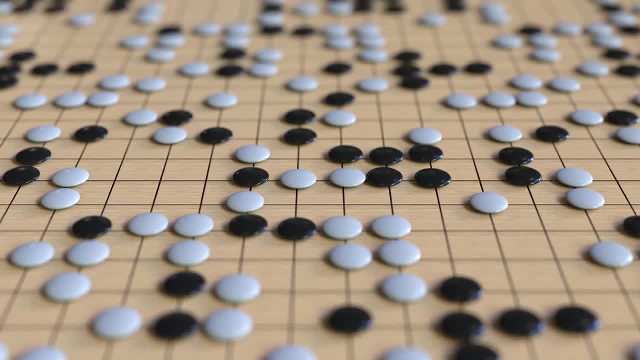 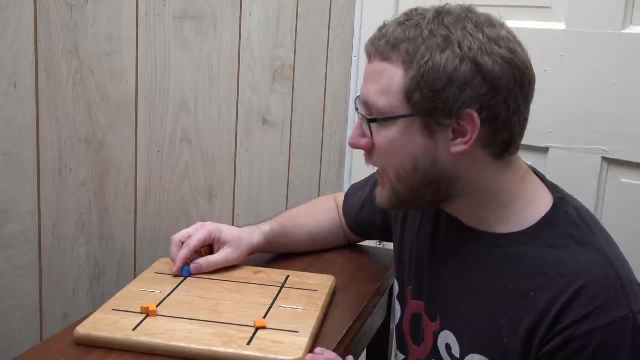 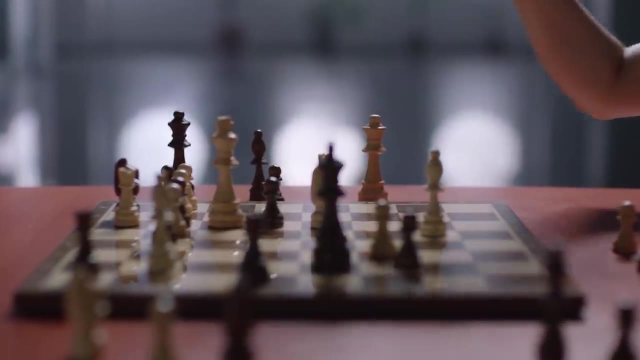 way With Go, you're grabbing territory by placing blocks And the only randomness is what your opponent's going to do. These games are high, high strategy, But you don't get a lot of surprises. So there's no randomness in chess, There's no randomness in Go. High strategy games, Kind of. 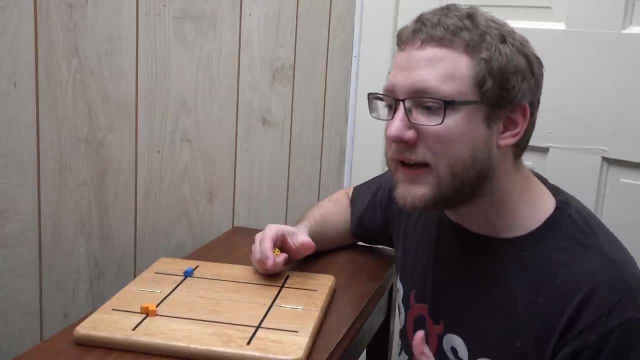 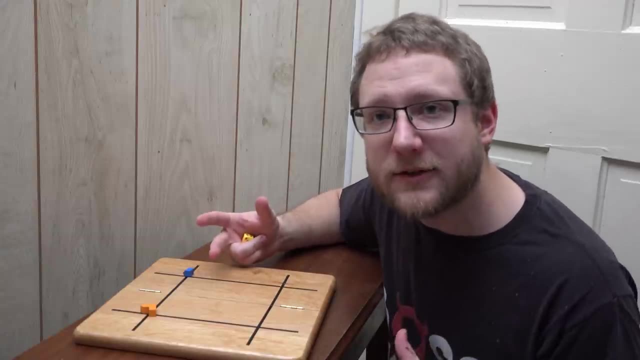 more of a fun generic game. When you can kind of throw those mechanics together, then you can create a strategy and you can make backup plans when things go wrong. do fun things, make interesting decisions. You can make those interesting decisions with a bit of randomness. So the dice, I'm going. 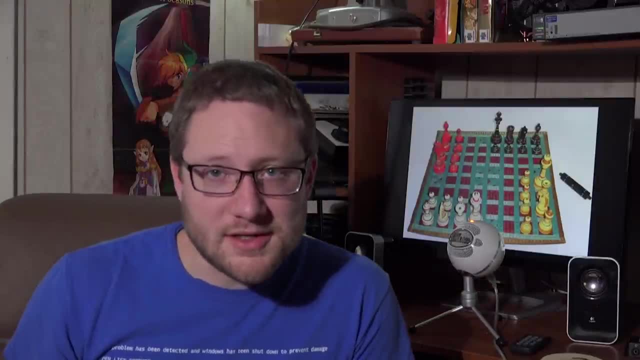 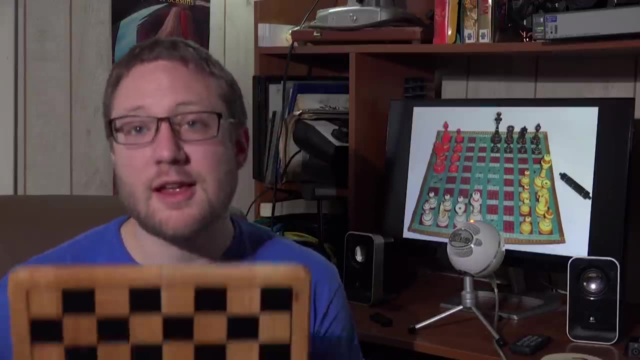 to have to make a die. I'm going to make the pieces. So I've been looking for some inspiration for making a board game with Iron Age tools, And the good news is it's very possible. actually, Good inspiration has been wood. This is a wooden checkerboard. Wooden checkers also give me another. 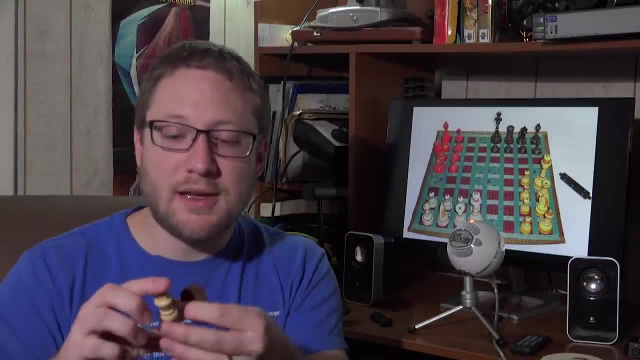 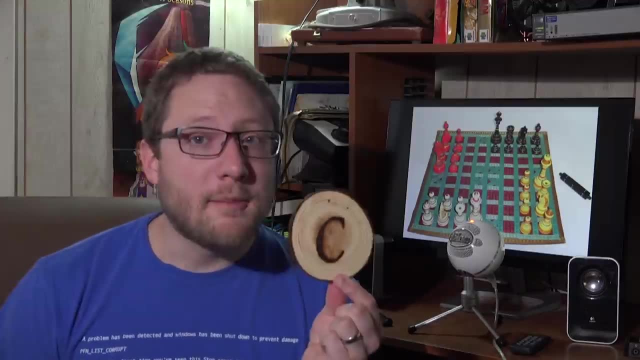 idea, Since really I'll be either whittling or doing something with the pieces. this is a king from a chess game. Wood would make a very good material to use for this. My tokens for the game will be smaller than this, but this allows me to take a saw which, thankfully, has been created. 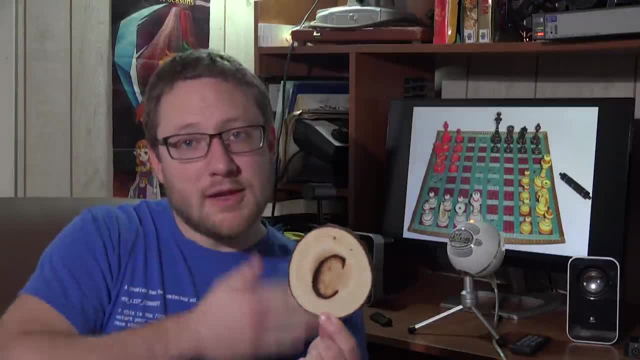 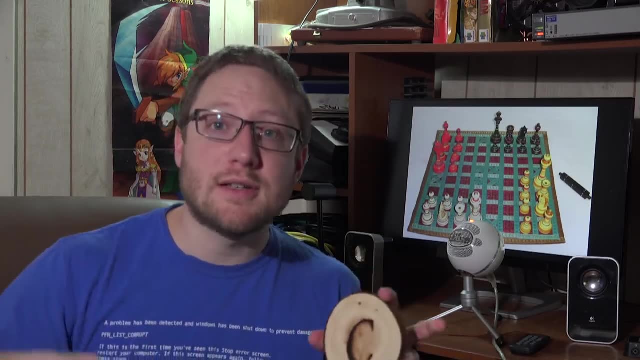 already by Andy and saw sections of a stick across to make kind of wooden coins. And these wooden coins can be wood burned to give them certain symbols And the symbols can differentiate them from other pieces. As a viewer of the show, I've always wondered. 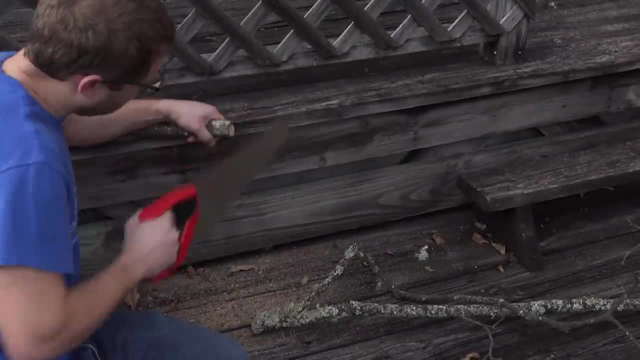 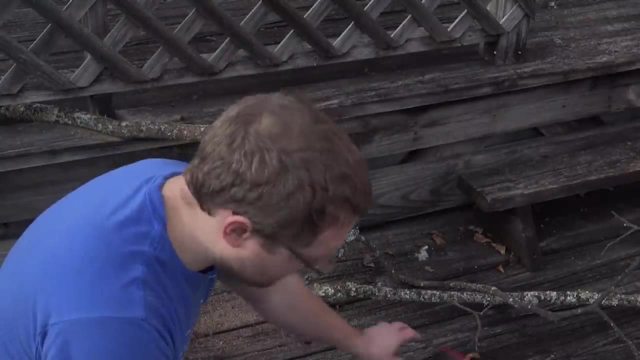 how long it actually takes to do these things, Like I always knew how hard it was watching the show. But when you do it, when you're like, oh, I'm just going to make this one scratch real quick. there is no real quick 20 pieces. Now I got to make a cube. What I'm going to try to do is use 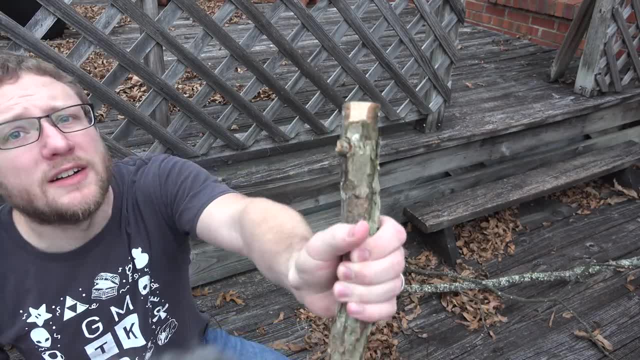 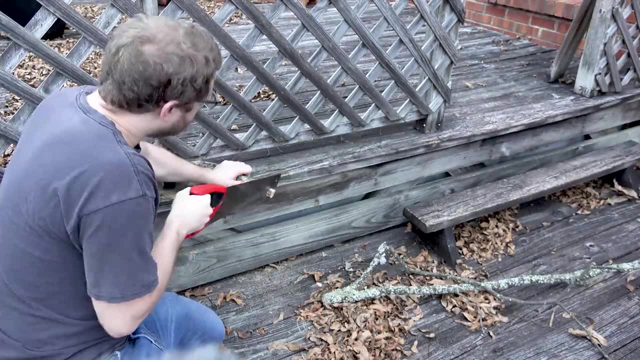 a saw to give myself a nice straight edge on each corner coming straight down. And then I will saw it down, And then I'll use my knife to whittle out the corners. All right, Not a cube yet. And then that should. 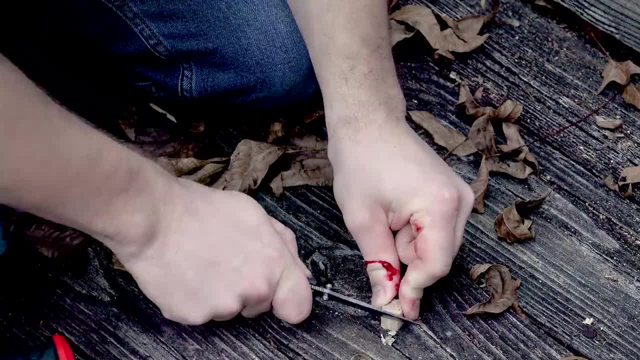 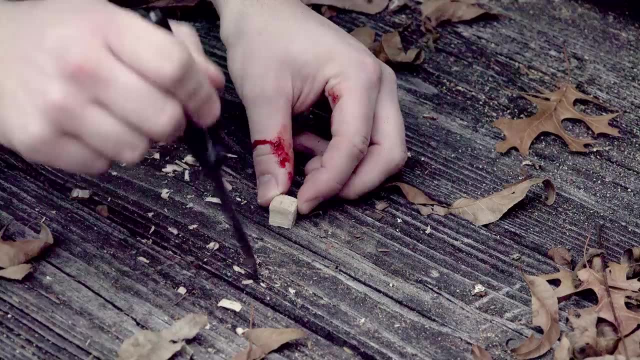 give me some sort of a dice that we can have as a randomizer, Evening it out. try to make it more of a cube. I guess I got to cut little notches for how much the die is worth on that side, So you. 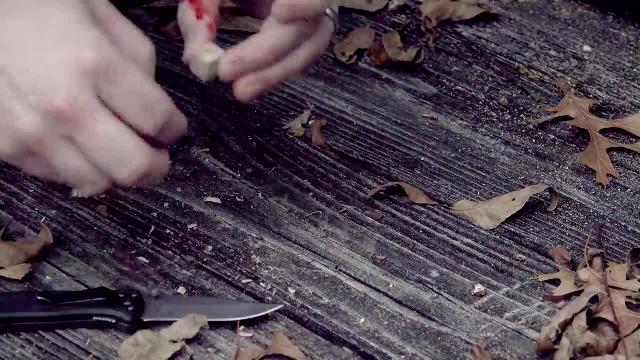 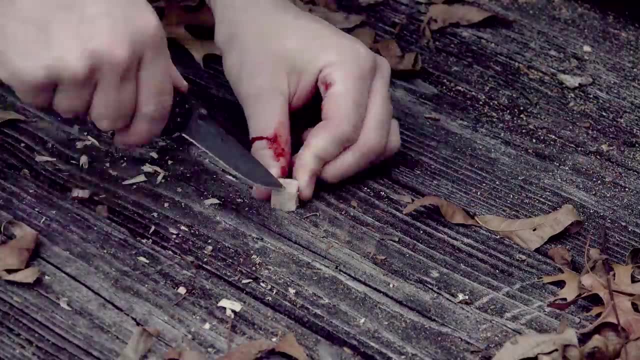 buddy, you're going to be one. I could use blood as paint, but I don't think Andy and his team would appreciate getting like a bloody dice. but that would actually be really convenient right now. Five, All right, Six, one. 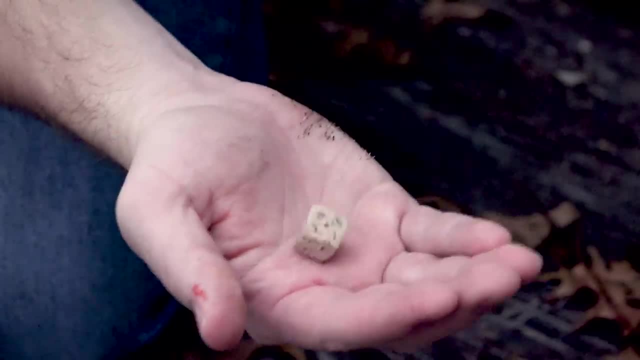 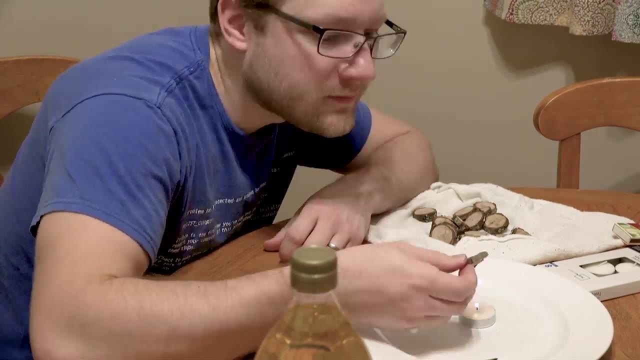 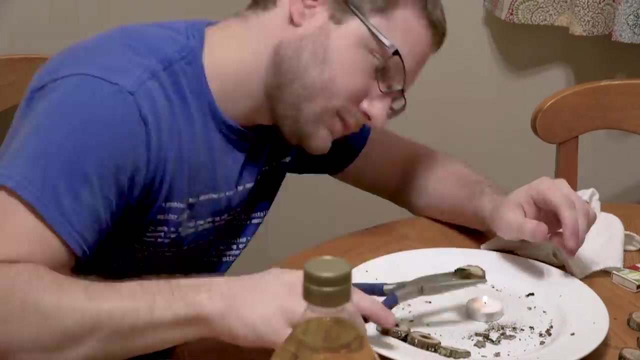 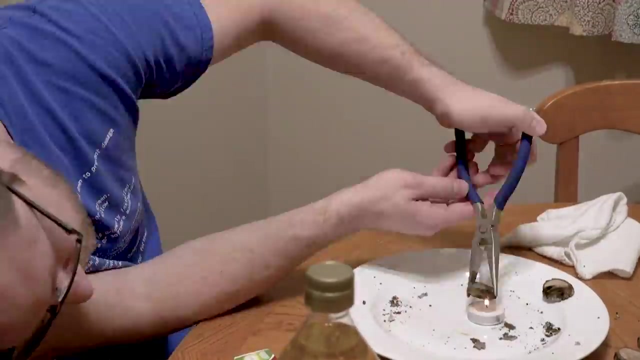 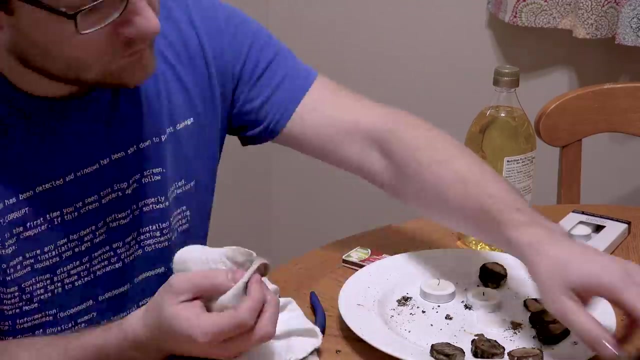 five, three, four. It's a dice, All right, So I've got my wooden pieces, Let's try this. Hey, we got a market, So staining it actually is removing the soot, So I'm just going to have to stain it. Stain them and see what happens. Some of them are turning out. 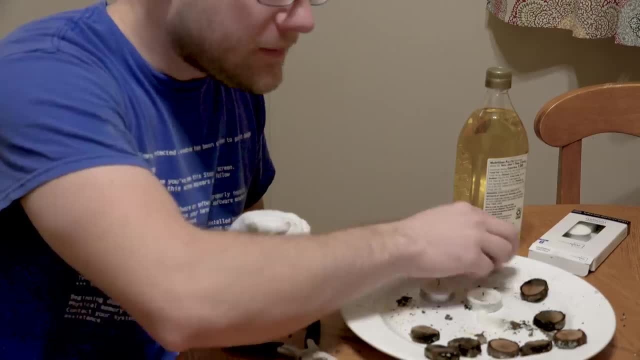 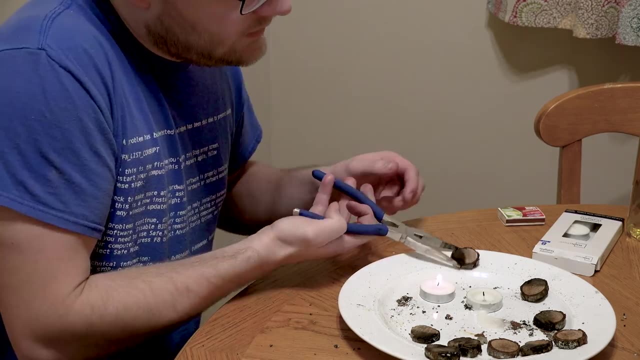 We'll see. This one still looks half and half. I might still go with this method: Oof, Oof, though That's been a lot of oof, A lot of work. Okay, That one's good, That one's good. 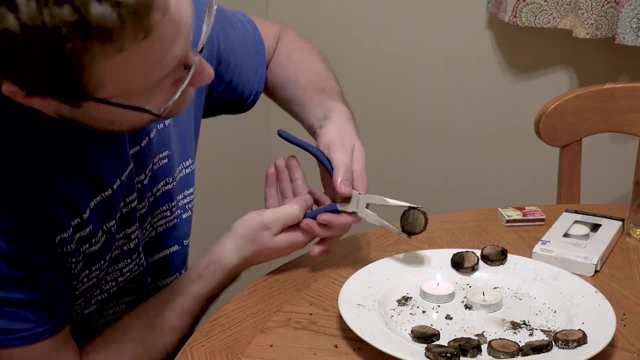 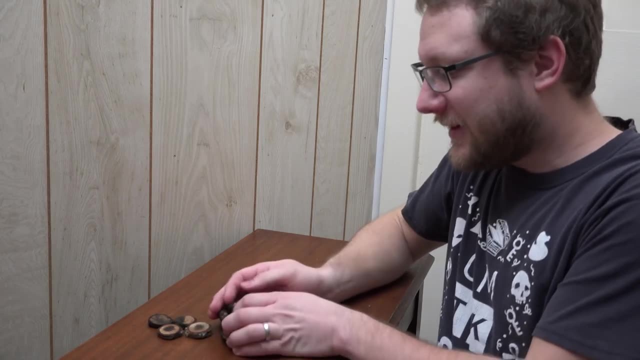 You've graduated to a black piece. You're just going to go the whole nine yards. So here we go. We got all the pieces here, Lots and lots of beautiful pieces you can touch. This is like a standard piece: the half. 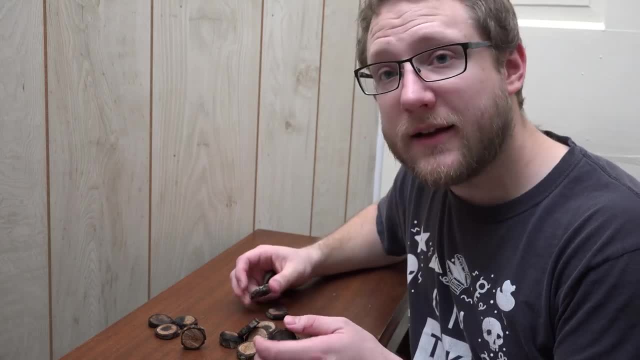 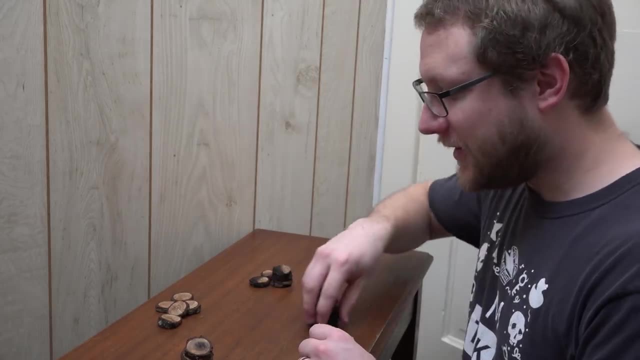 piece, dark piece, the one hit piece, That's it. So I've got all these different pieces here. That means everybody can have their own custom pieces to gamble in the middle. We have a randomizer and it works too. I've been rolling it over and over again to make sure that this doesn't roll. 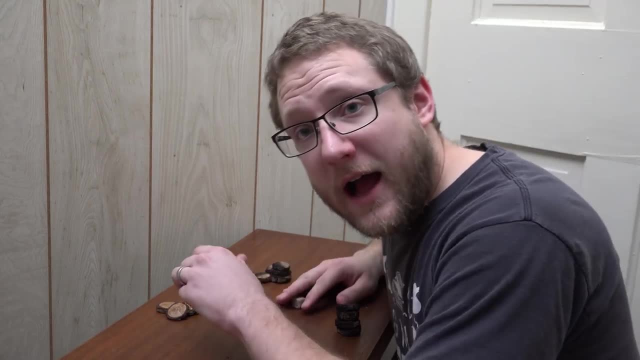 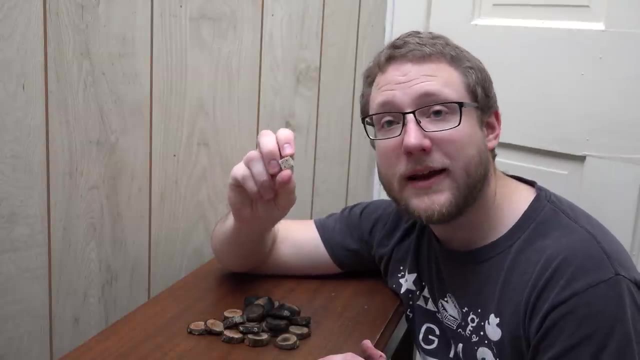 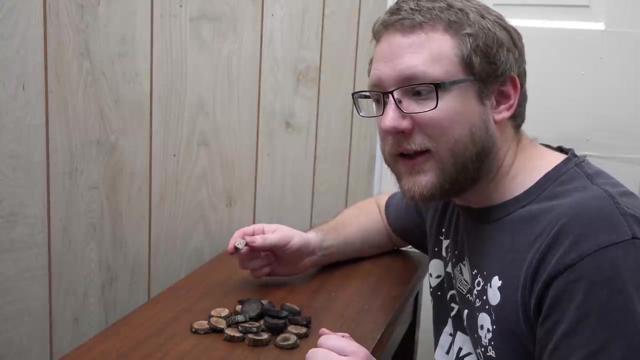 like a six every time I've got a game here. So I got to mail this to Andy. This took blood, sweat, no tears, though, to make. You can see why board games. in ancient cultures they were a lot of times buried with their board games and stuff, Or they carried them around a 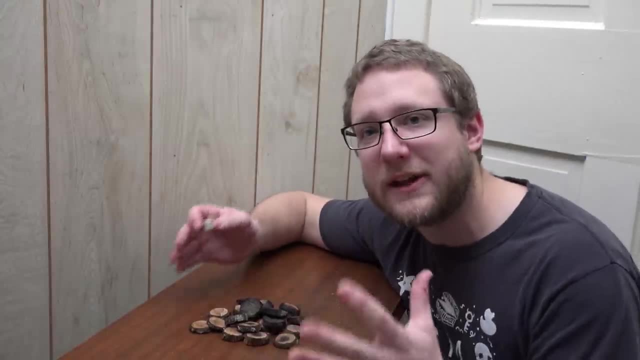 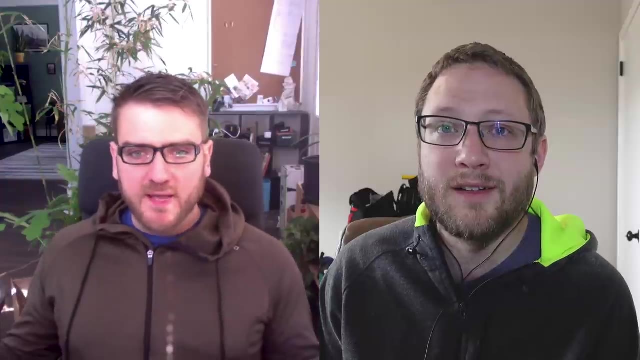 lot. There's a high social value to their games And one reason is because they were probably expensive. Like rich people probably had games And uh. so here you have an update on the project. Quite a lot of effort to get this uh thing built. 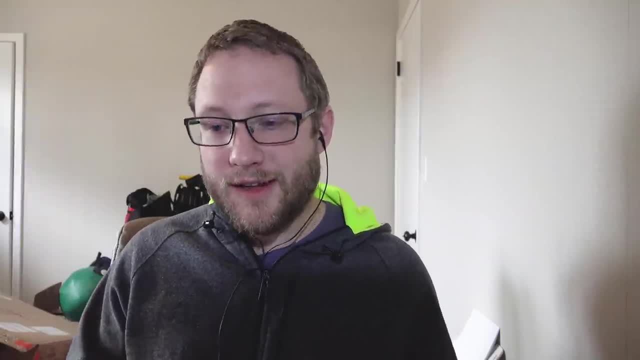 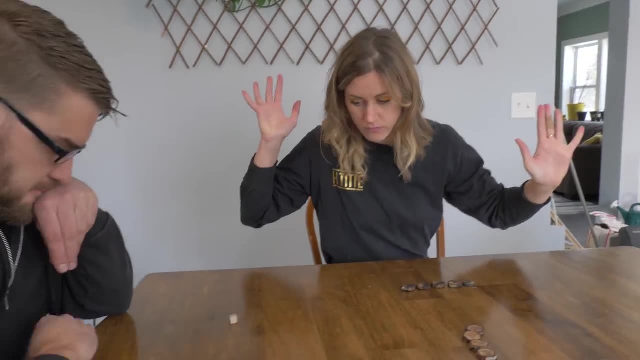 but I've got a game- uh, that should have tokens and a dice that you can roll, that we can play this game, And so what you'll do for the game is the first player you'll roll to see who goes first, And the first player will pick an amount of tokens to bet. You can bet up to one token. 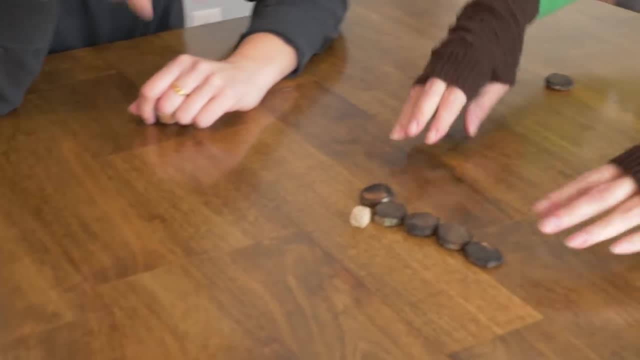 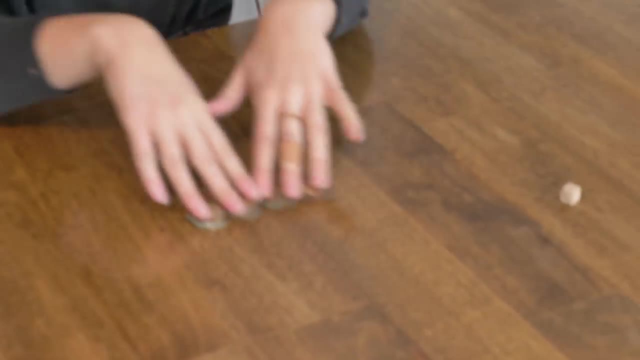 all the way up to five tokens, And if you bet five tokens, the player next to you rolls to try to take your tokens. If they roll a number higher than the amount of tokens you bet, then they get to keep all of your tokens. If any player gets all of another player's, 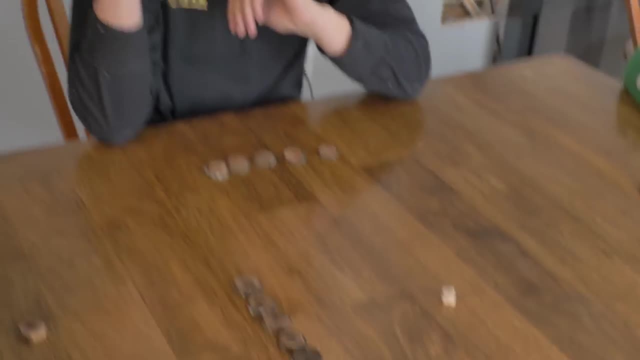 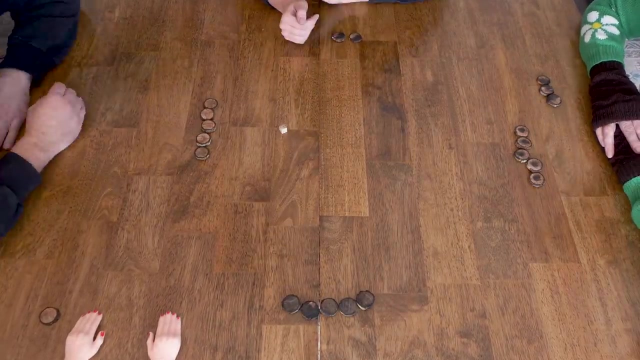 tokens, they lose. but you're trying to make sure that another player in the game doesn't get five of another player's tokens. that you want five and other players tokens. If you do that, you win the game. Everybody else loses. There's a negotiation segment too. If, for whatever reason, somebody 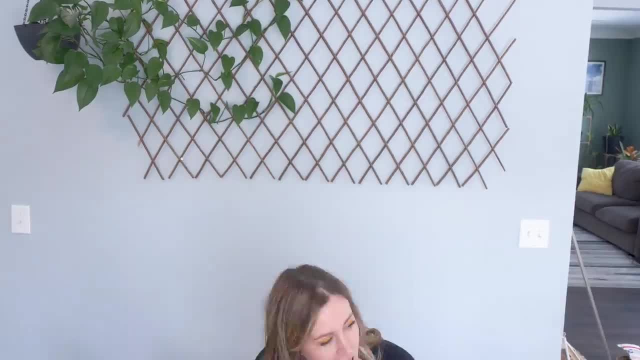 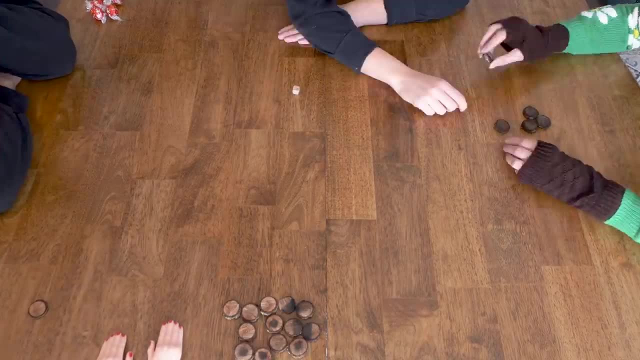 rolls and tries to and wins this pot. what they could do is try to sweeten the deal for both of them and say, okay, I want to make this. I want to trade instead for these particular tokens. If the person agrees that trade happens. 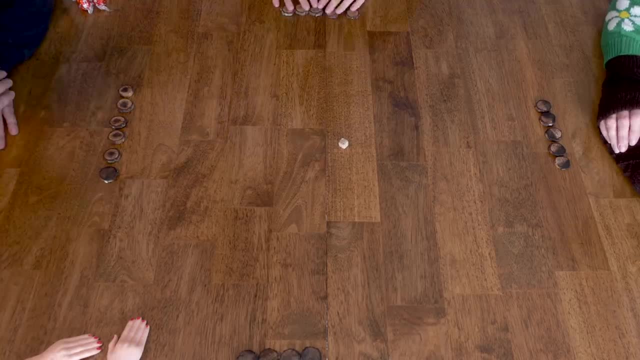 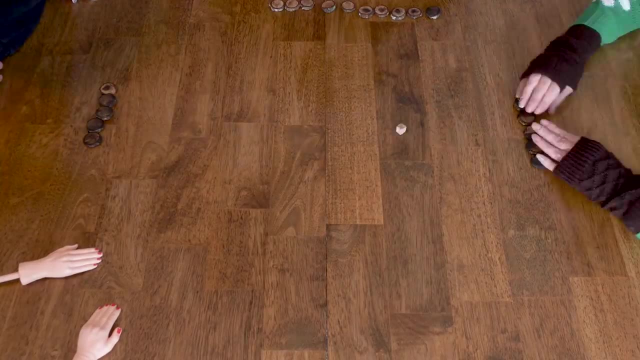 if they disagree, they do not win the pile, They've lost it. So, taking the game Adam sent we play, tested it a few times. It felt like it had the basis of a pretty decent game, but we found that it had some issues with the strategic aspect. after, 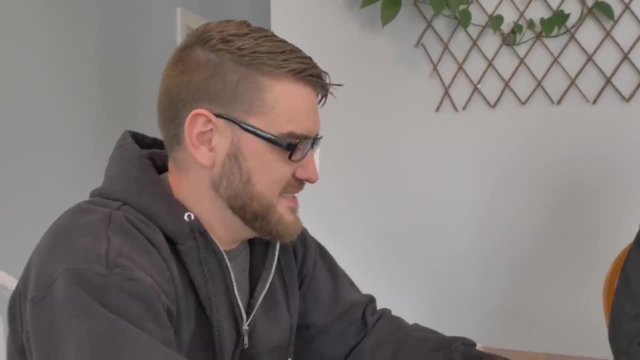 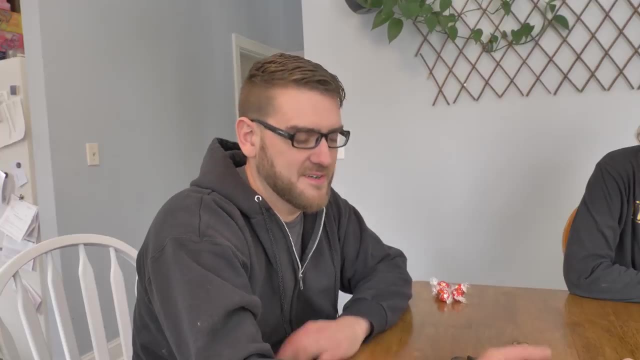 a few rounds. So I think my biggest criticism is that it basically goes down to who can roll six. first It's all the incentive is to, if you have enough pieces, put them all in There, cause then the odds are in your favor, Uh, and then it's just a matter of who rolls six. 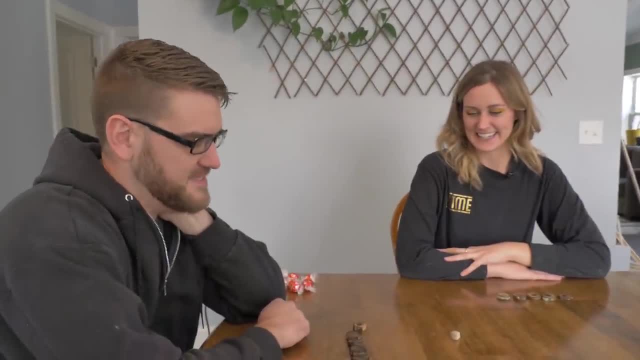 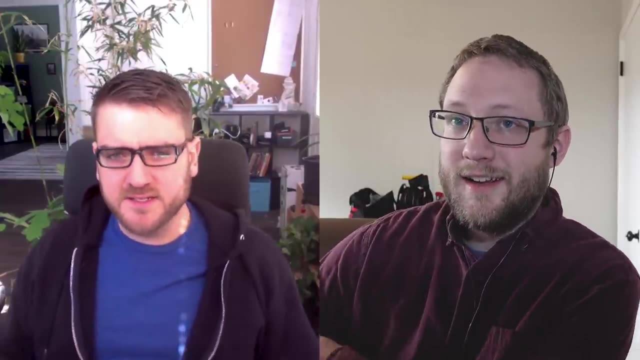 often. I don't think there's been like any incentive to like try and make a deal. I relayed my experience with the first draft of the game to Adam and gave him an opportunity to try and develop the game a little further and see if he could address. 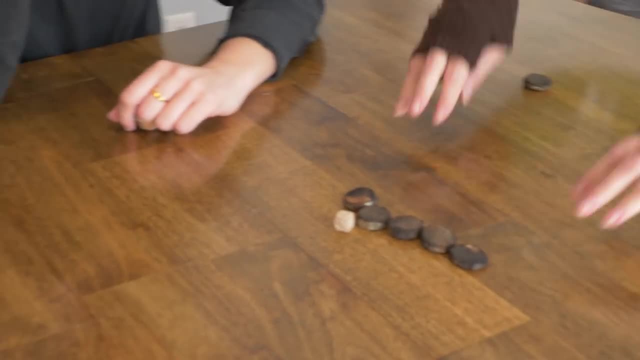 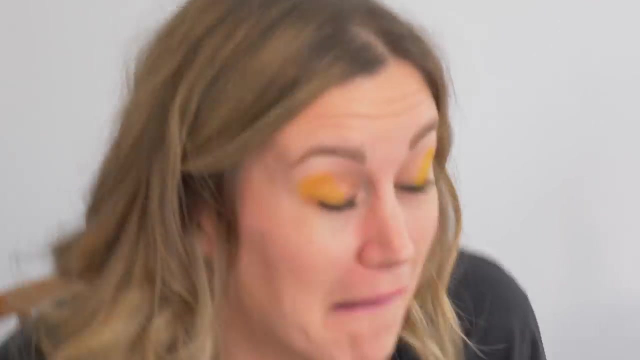 some of these shortcomings. One additional issue I ran into is that, while Adam's medallion tokens were a decent primitive solution, it ended up being a little difficult to easily identify and differentiate, So I thought I would remake them a little bit more unique. 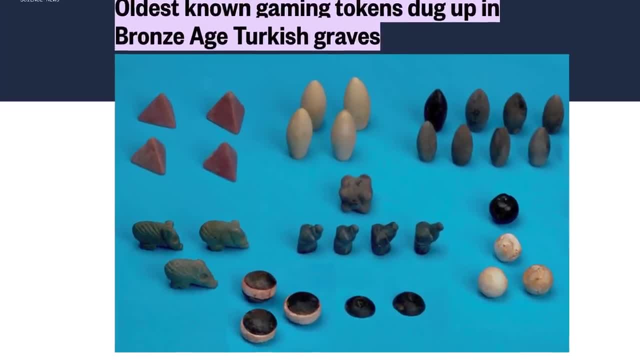 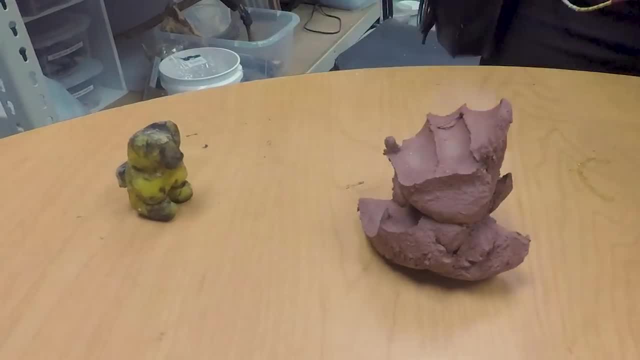 in a metal. For inspiration, I looked at some of the earliest game tokens that have been found, like these triangulator pyramid shapes and various animals, So I also used this opportunity to recreate the mold- Annalise made way back- of a small little lost wax statue of my cat. 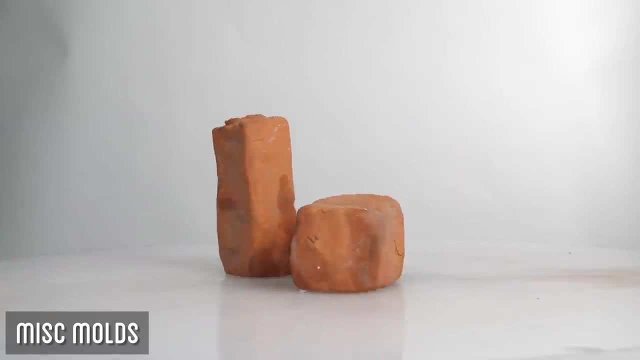 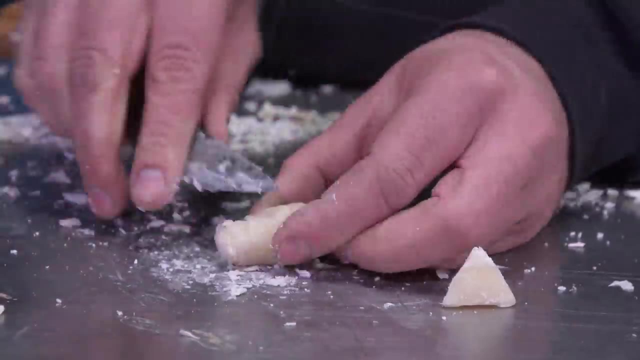 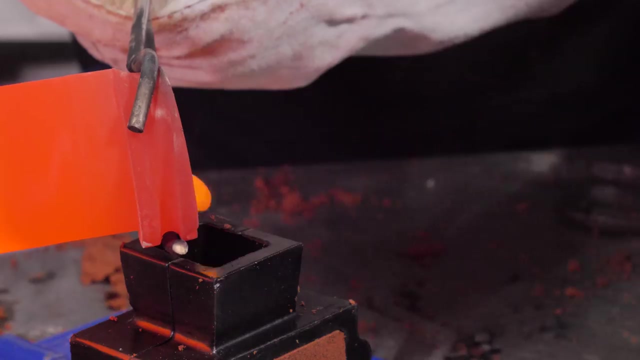 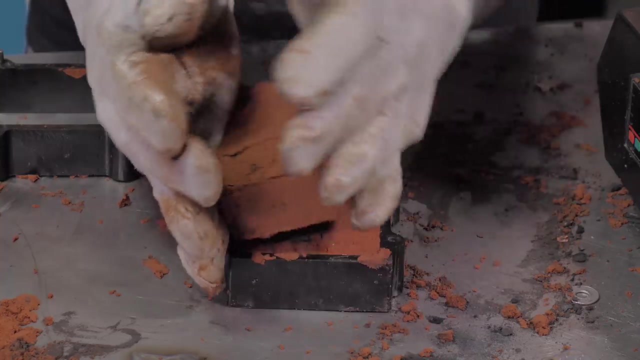 Dobby Never actually cast that but did sell it on the auction. So somebody out there does have this original mold. So to make these I first carved them in wax, Then I sandcast a set of five of each token in two different metals: bronze and tin. 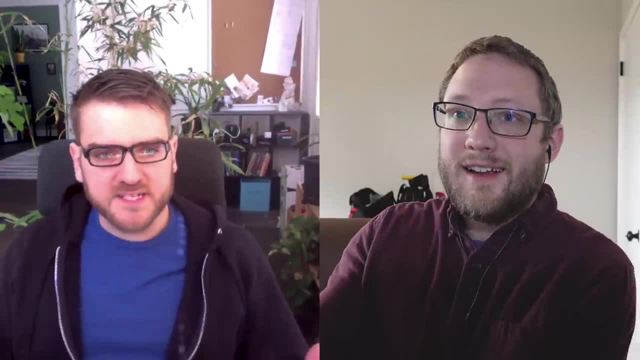 Then I sandcast a set of five of each token in two different metals, bronze and tin. Hey again, Adam. So I play, tested the game and kind of let you know a few thoughts on it, a few issues I saw possibly in it. and yet you've had a chance to kind of 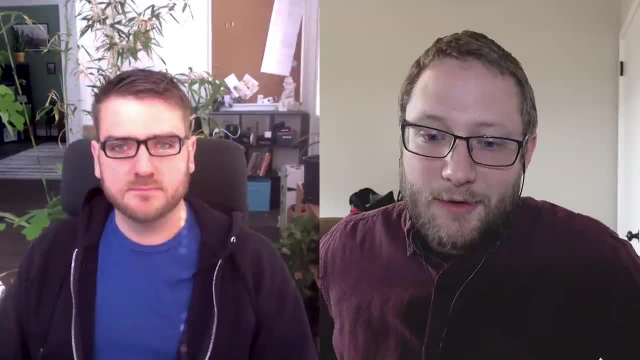 adjust it a little bit, All right. So what are the new rules? What I did is I went and I changed a lot of the rules and play tested a lot of the rules. A lot of the concerns were things like the communication wasn't happening that I planned. 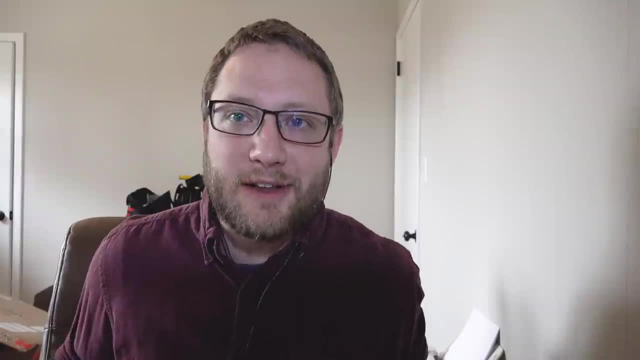 to happen and the randomness was taking over, and that's not the kind of game we wanted to make. So there's going to be more than one way to win. The original way is to get five and another player's tokens. That's still a way to win, But also you're going to get five and another. 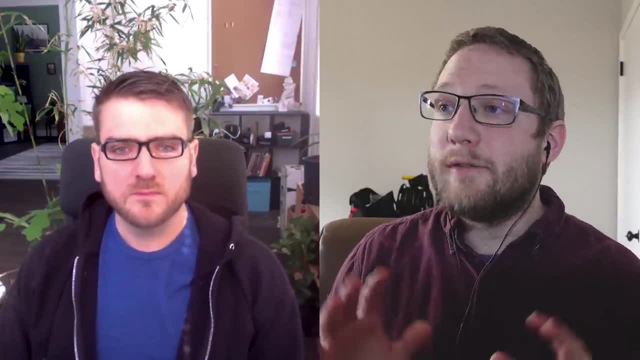 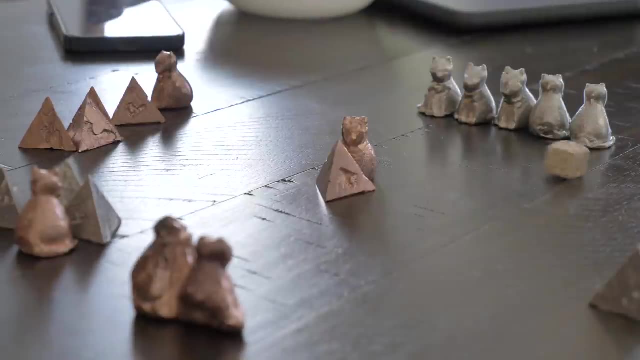 player's tokens. That's still a way to win, But also you can have two of every single player's token, and that includes the player. if someone gets eliminated, that includes their tokens too. two of all the tokens in play. The max bet is now three, So five was too safe of a bet. You have a. 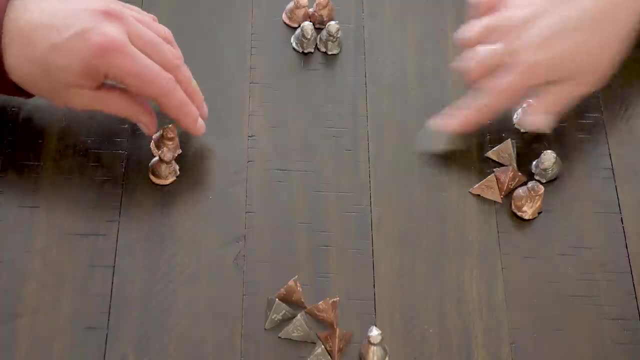 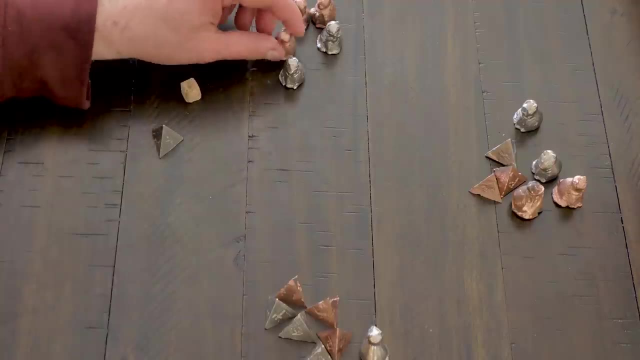 little less control over if you keep your tokens or not. Instead of negotiating. and when you want to pot, everyone has to trade at least one token every round. So when you get back to the original player, you have to do another trade- at least one trade of one token with someone else. So 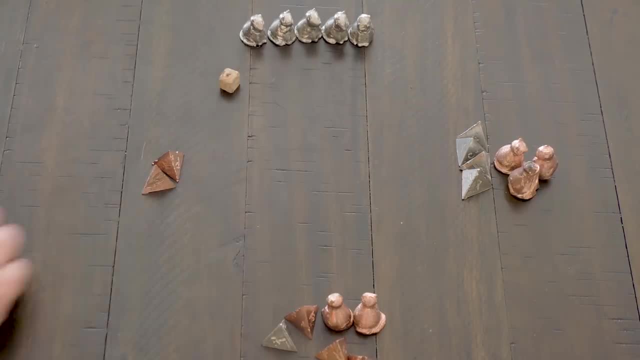 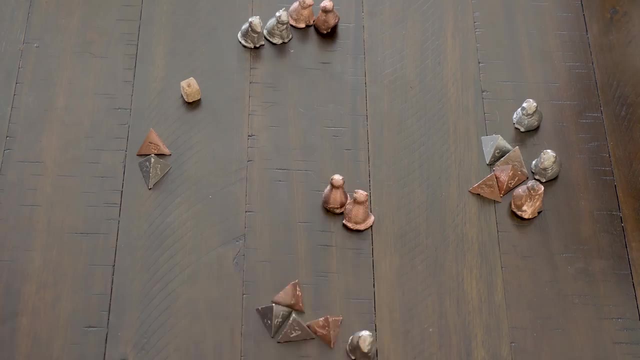 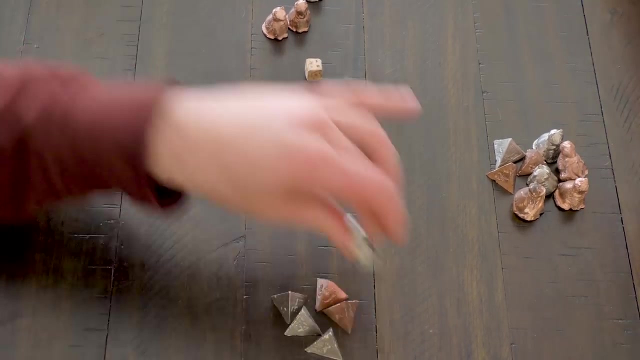 if that trade, if someone's eliminated, you'd no longer have to do the trading round. If you bet only one, you have the option to reverse the turn order. So instead of going to the player to your left, it can go now go to the player to your right. We were almost to the final version of the rule. 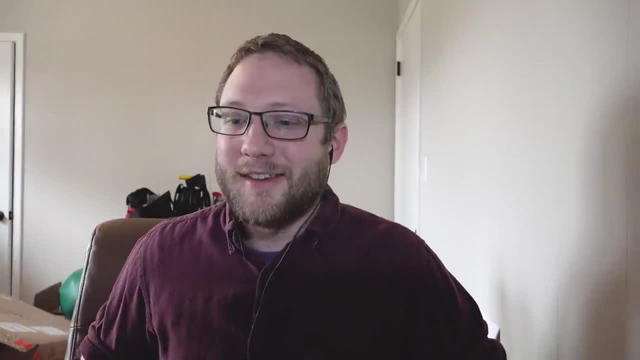 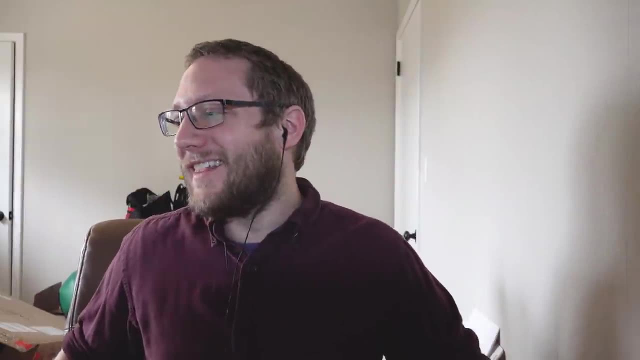 and I play- tested it with my son originally. He's playing it- and in the middle of the game goes: this game's actually fun, And I was like: oh okay, I didn't know that the other one wasn't. So I think we're on the right track, at least After having the chance to play with the new revisions. 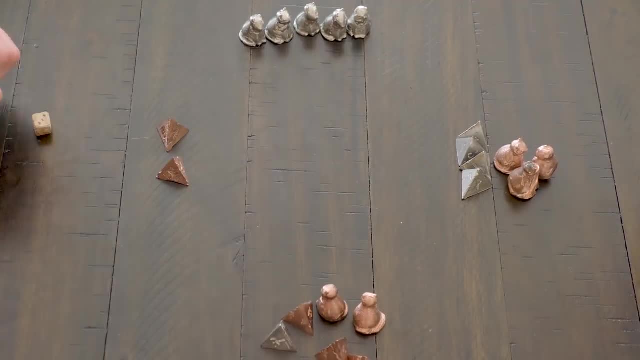 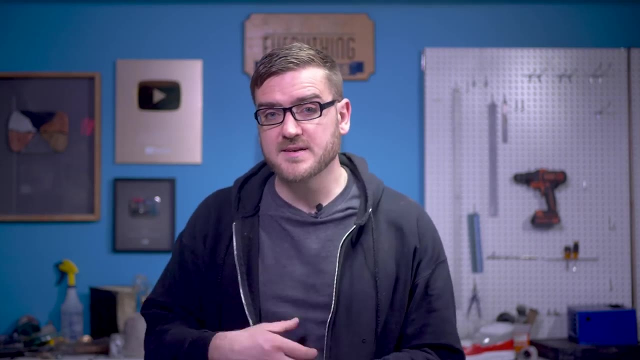 it was a lot more enjoyable and a pretty fun game. Our top $75 supporters on Patreon will be getting their own 3d printed version of the game. I'm going to be sharing the rules and everything with everybody. Try it out. Game development- It's kind of an ongoing evolution. Chess started out in. 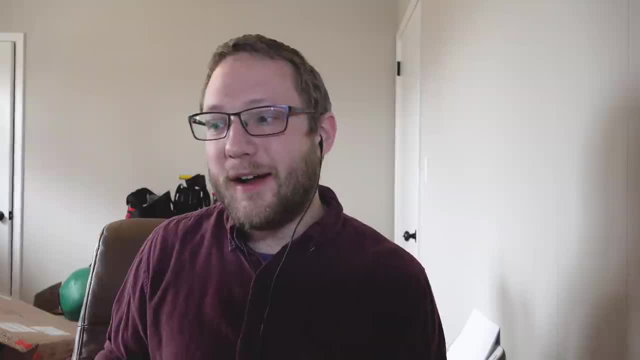 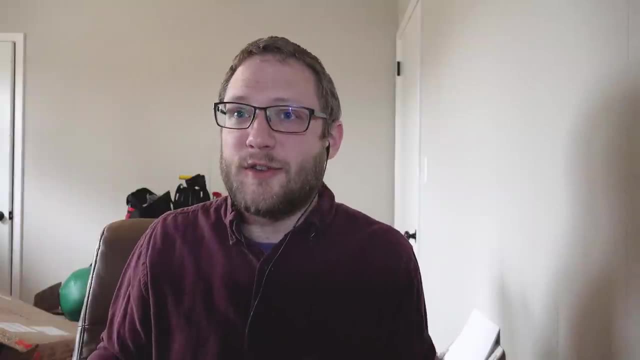 India and it had like a version in Rome and chess was really four players. Then I had a two player version And then eventually in the middle ages somebody said: what if the queen could just do all the moves? And that's called mad, mad queen's chest, And that's actually the 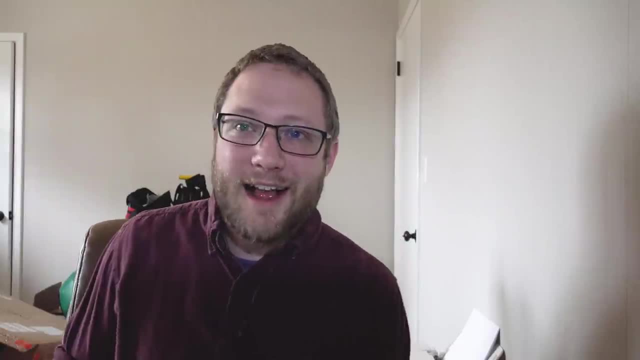 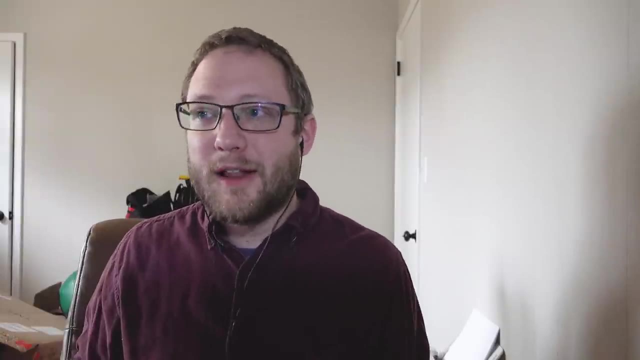 version of chess we play today. So games just take a long time to iterate. I think the iterations we've gone through have definitely improved it And there's a chance that, you know, maybe some of the viewers will see a thing and they're like: you know what? what if we added this rule or tweak? 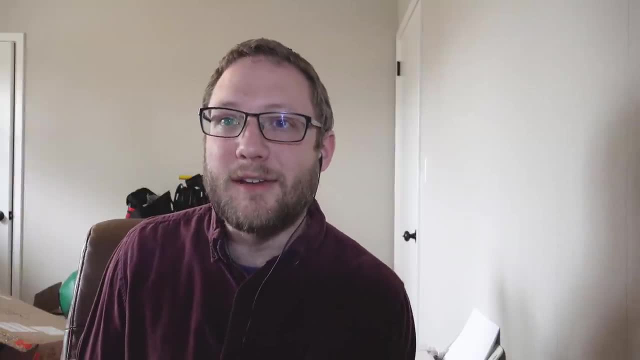 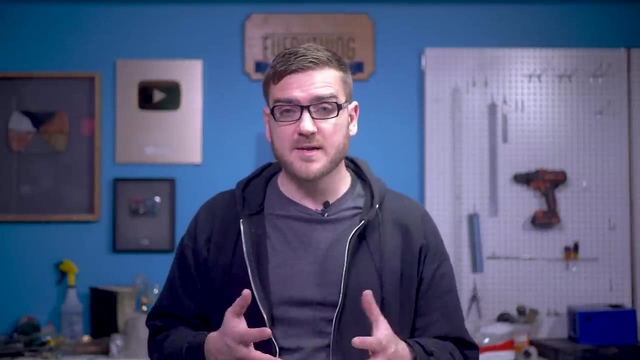 this rule and kind of improved and perfected the game. I'm excited to see if anybody's got something to say about that. So it'd be interesting to have a bunch of people play this game and come up with their own ideas for improvements to it. Try out the game. Let me know in the comments. 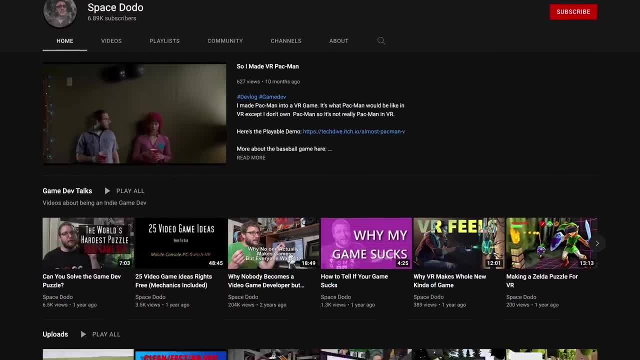 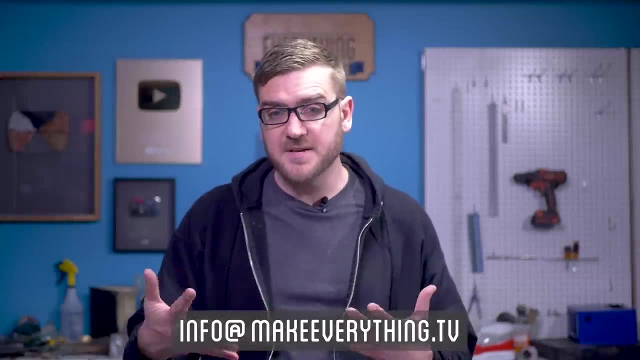 let me know your thoughts. Be sure to check out Adam's YouTube channel, Space Dodo, where he explores the topic of game development in a variety of other ways. We have a couple other guest videos coming up, but if you have your own idea that you want to pitch to us, shoot me an. 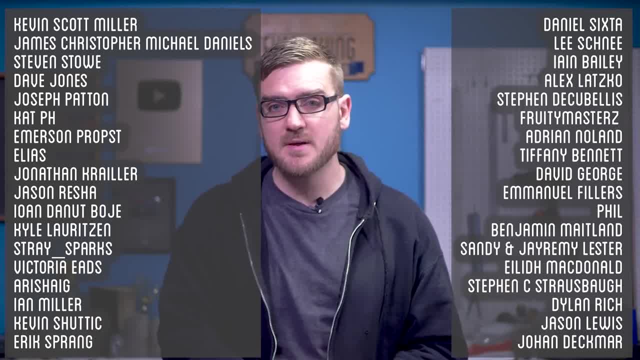 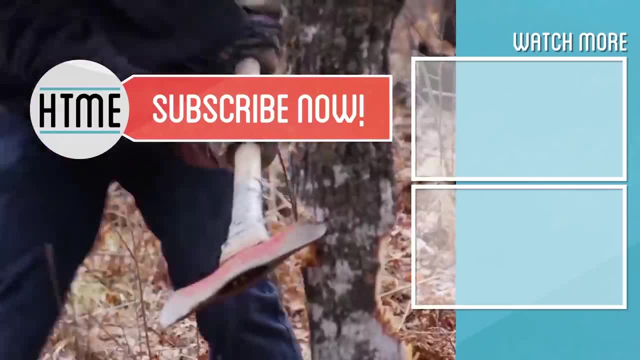 email. Thanks again for watching. Thanks again to all of our supporters on Patreon. Got some new content coming up, So stay tuned for that. If you enjoyed this video, be sure to subscribe and check out other content we have covering a wide variety of topics Also, if you've enjoyed. 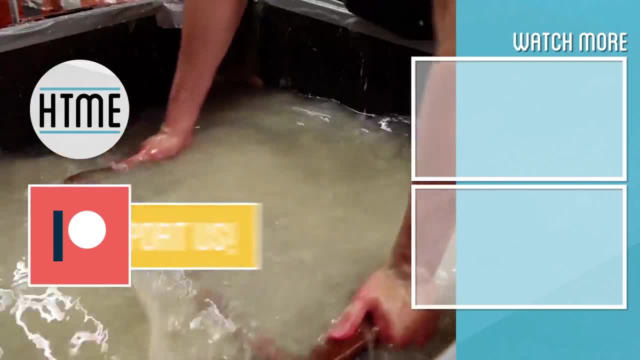 these series. consider supporting us on Patreon. We are largely a fan funded channel and depend on the support of our viewers in order to keep our series going. Thanks for watching.